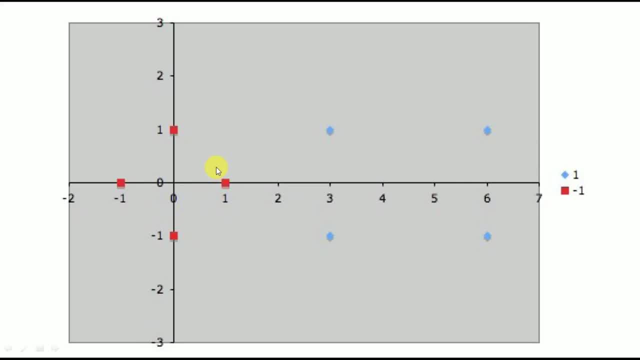 data point which is nearest from negatively labeled data points and these two are from positively labeled data points. So you can say that this is 1, 0.. We will label this one as S1 and this one is S2. that is 3, 1 and this is S3.. We will say it as 3 minus. 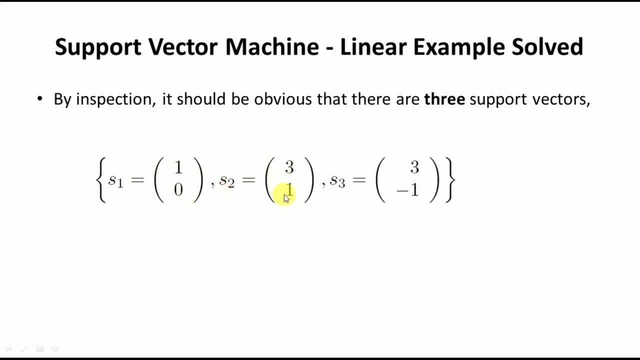 1.. So S1 is equivalent to 1, 0, S2 is equivalent to 3, 1 and S3 is equivalent to 3 minus 1.. So this is the next step, what we need to perform. So, after this particular thing, 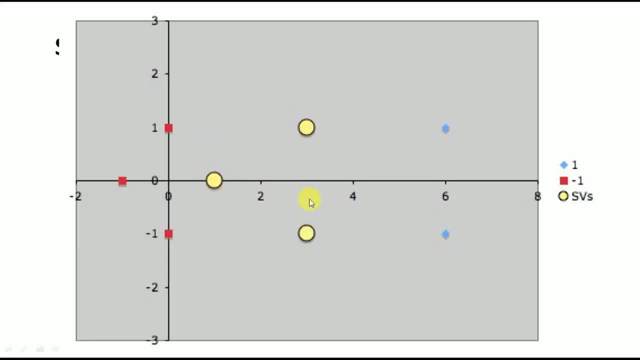 this is how actually the graph will look like: This is the S1, this is S2 and this is S3.. This particular point is from negatively labeled data set and this is from positively labeled data points. Now, whenever you write a equation for the hyperplane this side, it will be equivalent. 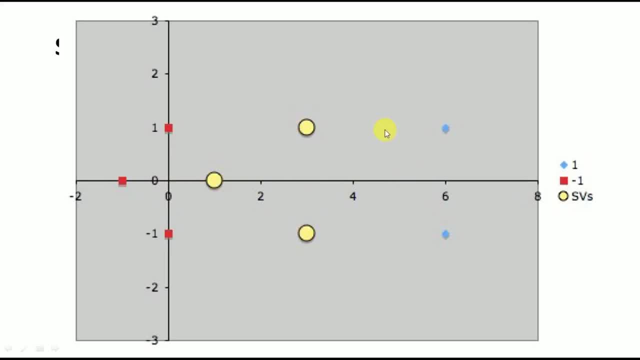 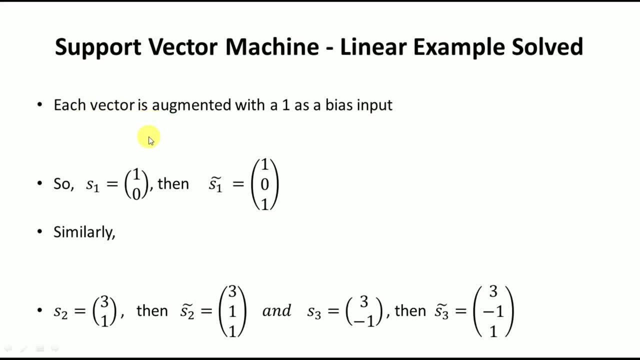 to minus 1 and this side it will be equivalent to plus 1.. So that is how actually we used to write the equation. Now, what we do here is, for each vector, whatever the three data points we have identified, we used to augment one as a bias input. So that is what actually. 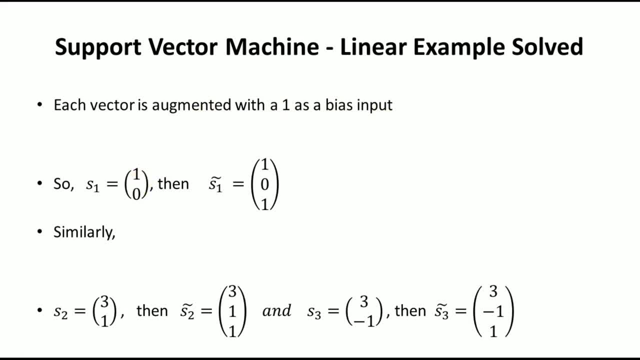 we used to do before we continue with the procedure. So first, OK, S1 is equivalent to 1, 0.. This S1 is converted as 1, 0,. 1, that is, 1, will be added as a one. 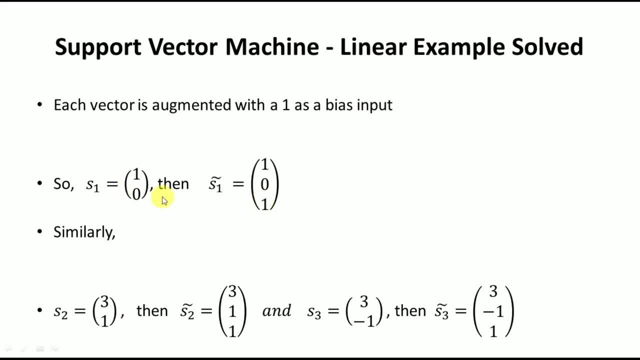 more dimension to this particular S1.. That particular dimension is nothing but a bias. Similarly, S2 is 3, 1.. 1 will be added to it. It will become 3, 1, 1.. And S3 is equivalent. 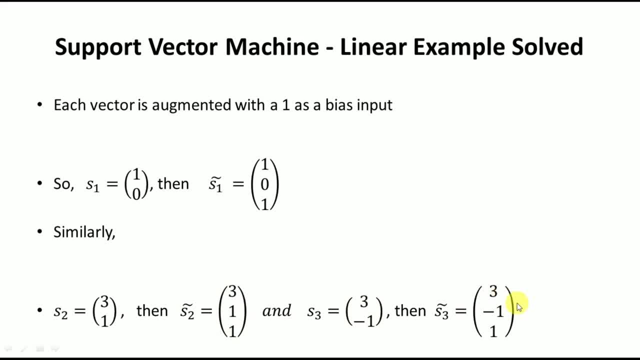 to 3 minus 1.. once we add 1 to this one, it will become 3, minus 1 and 1.. So just to differentiate these two data points: S1 is the original one and S1 is the single data. 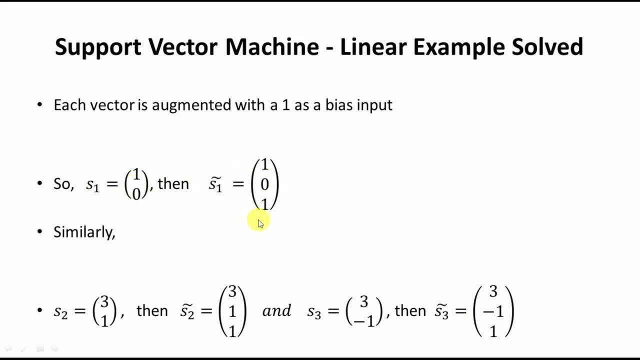 1 and S1- tidal is the data point after adding 1 as a bias to it. So similarly, S2- tidal and S3- tidal. here Here we have three data points which are near from either side of the classes. So what we need to do here is we need to calculate three variables, that is, alpha 1, alpha 2, alpha 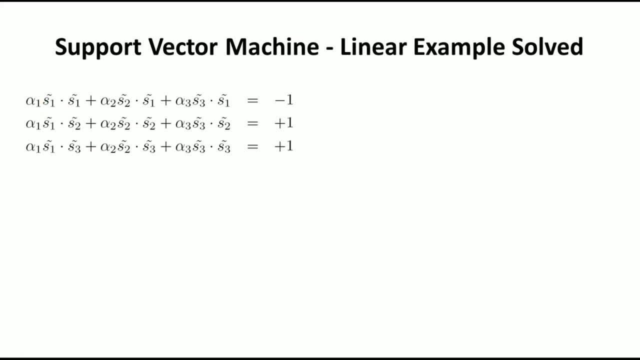 3, which will be used to calculate the weight vector. So if you want to calculate alpha 1, alpha 2, alpha 3, these are the equations we need to use. Depending on the number of nearest data points, these particular equations will change. So in this case we have three nearest data points. 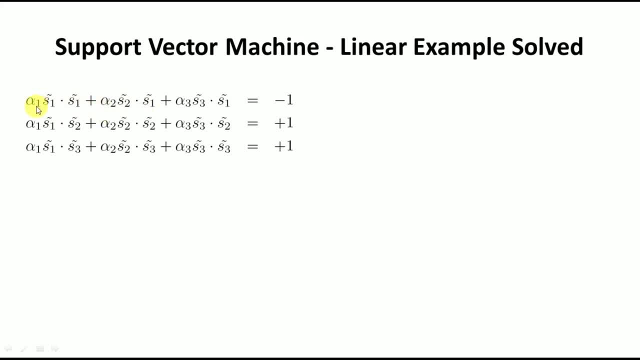 So we need to calculate three variables, that is, alpha 1, alpha 2, alpha 3.. Now the question is how to calculate it. So if you want to calculate alpha 1, we can use this particular equation, that is, alpha 1, alpha 2, alpha 3.. So alpha 1, S1, S1, plus alpha 2, S2, S1, alpha 3, S3, S1.. So if you 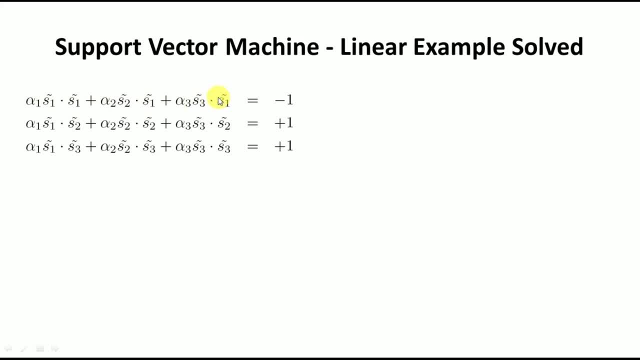 this particular equation. in this equation, S1, S1 is common and S1, S2, S3 are used for calculating or writing this equation and this one, S1, is common, So S1 is present on what side? S1 is present on the negatively labeled data sets. 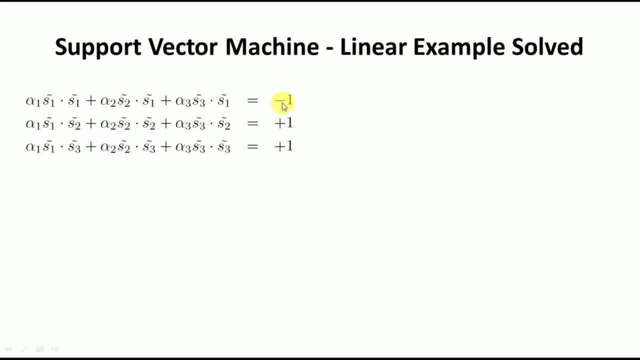 So we equate this particular equation to minus 1.. Similarly, alpha 1- S1- S2, alpha 2- S2- S2 plus alpha 3- S3- S2.. So in this case S2 is common. S2 is present on the positively labeled data set. So 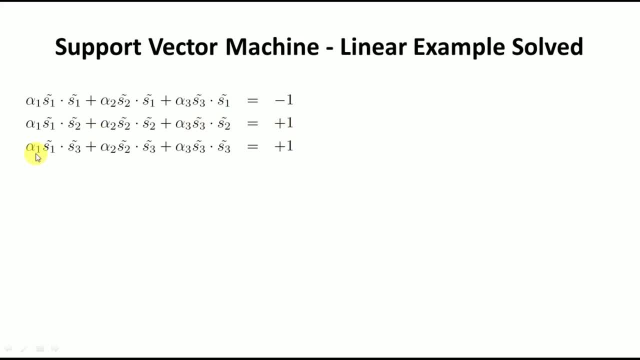 we need to equate this equation with plus 1.. Similarly, alpha 1- S1, S3 plus alpha 2- S2, S3 plus alpha 3- S3, S3.. So in this case, which one is common? S3 is common. Again, S3 is present on the 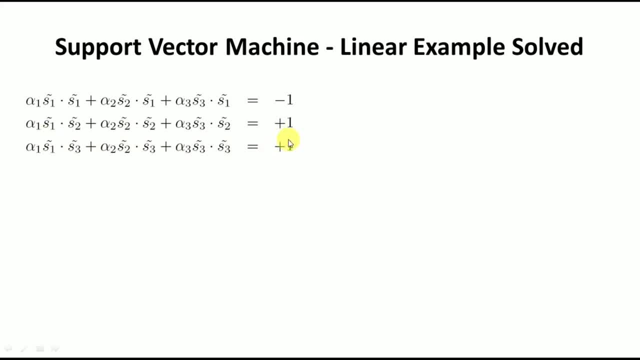 positively labeled data points. So we used to equate it to plus 1 here. Next, what we need to do is we need to put the values of S1, S2, S3 in this three equations. We will get these equations here Now, once you get this particular equation. so what we need to do is we need to perform the. 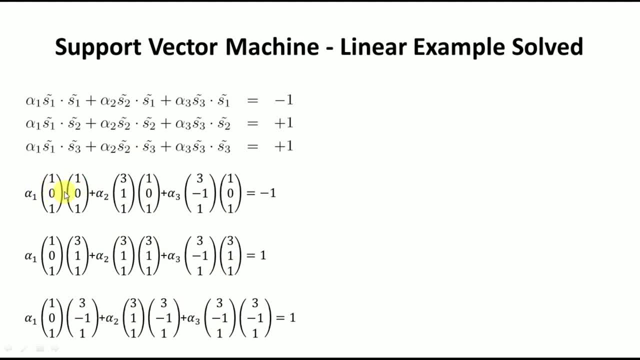 optimal. we can say that operations over here arithmetic operations. These are the two. we can say that the vectors. So we need to perform dot product between these two vectors. Between these two we need to perform the dot product Like 1 into 1, that is, 1, 0 into 0 is 0,. 1 into 1 is 1,. 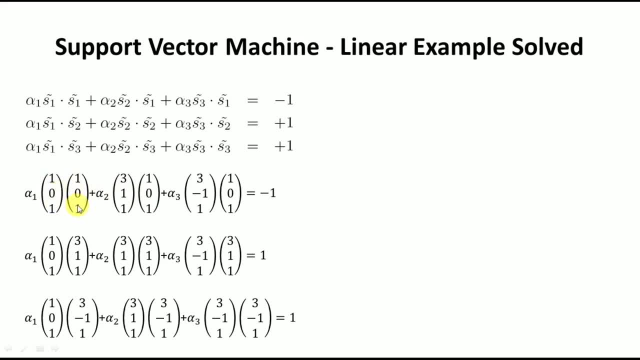 that is 1 plus 0 plus 1.. So that is the answer for this particular dot product. Similarly for this one: 3 into 1 is 3,, 1 into 0 is 0,, 1 into 1 is 1, that is 3 plus 0 plus 1.. Similarly, 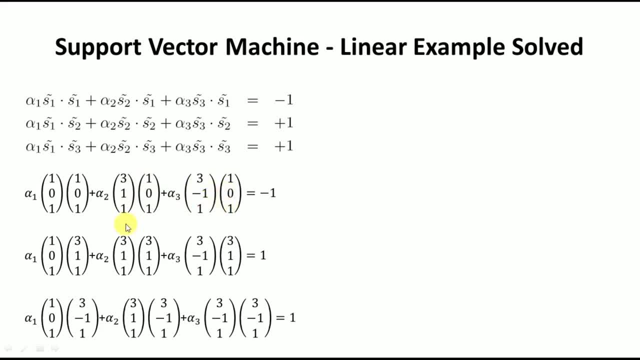 3 plus 0 plus 1.. With the same note, we can calculate or we can simplify these two equations also. We will get something like this: that is alpha 1, 1 plus 0 plus 1, alpha 2, 3 plus 0 plus. 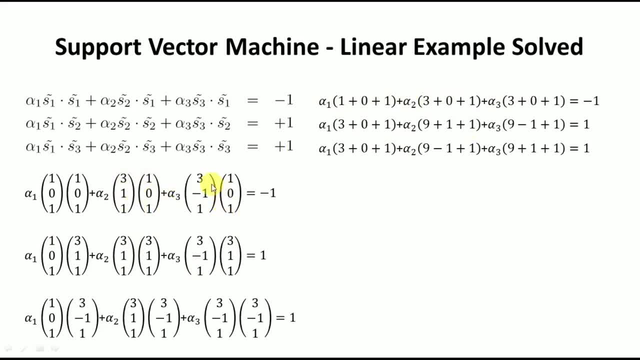 1, that is 3 plus 0 plus 1, and alpha 3 is equivalent to 3 plus 0 plus 1.. So this is the first equation. With the same note, we will be getting the second equation here and then the third equation. So 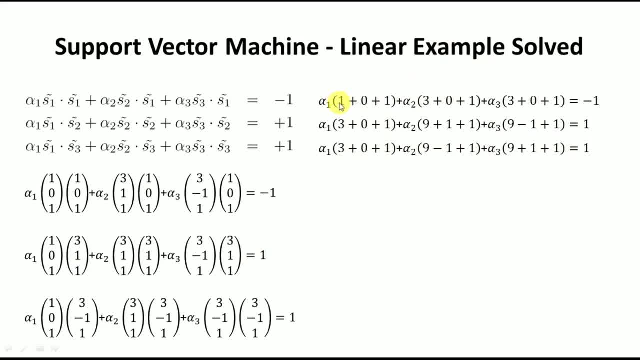 once you get these three equations, we need to simplify it again. that is 1 plus 0 plus 1 is 2, 2 times alpha 1 plus 4 times alpha 2 plus 4 times alpha 3, which is equivalent to minus 1,. 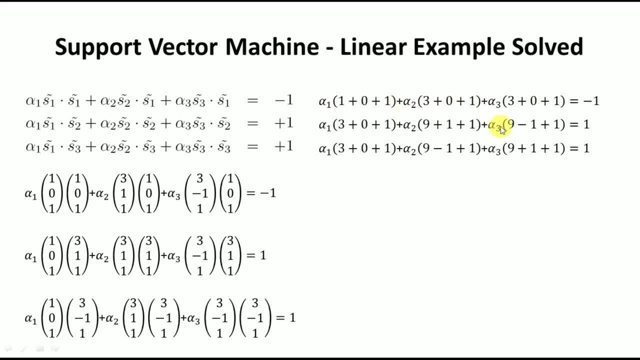 4 times alpha 1 plus 11 times alpha 2 plus 9 times alpha 3 is equivalent to 1,. 4 times alpha 1 plus 9 times alpha 2 plus 11 times alpha 3 is equivalent to 1.. 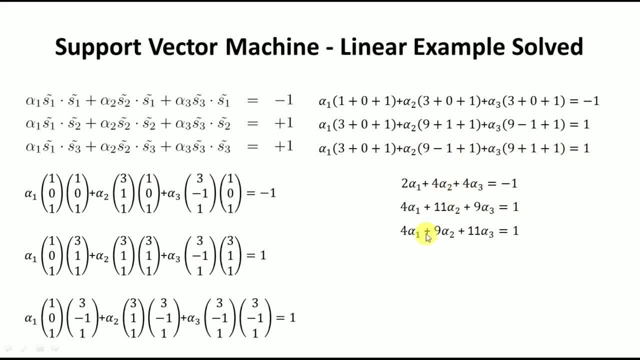 So, once you get these three equations, what we need to do, We need to simplify these three equations so that we will get the values of alpha 1, alpha 2, alpha 3.. We have 3, equations, or simultaneous equations. along with that, we have three variables. So definitely we 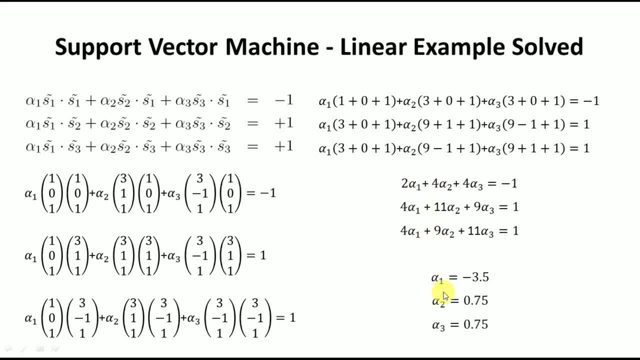 can easily solve these things, and then we will get the values of alpha 1, alpha 2, alpha 3.. So once you solve it, you will get: the alpha 1 is equivalent to minus 3.5, alpha 2 is equivalent. 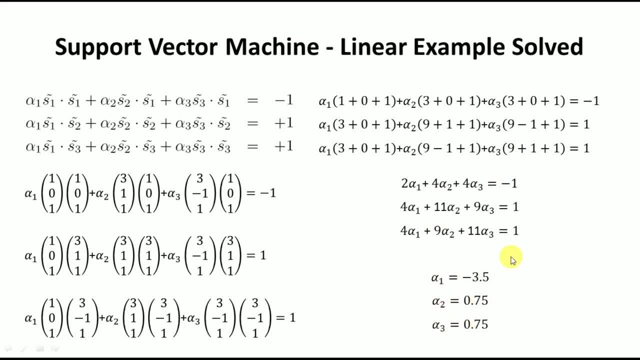 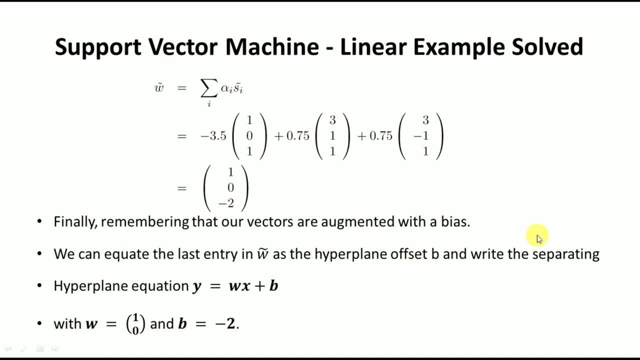 to 0.75, alpha 3 is equivalent to 0.75 in this case. Now, once you get three values of three variables, what we need to do is we need to calculate the weight vector, that is, w cap or w tidal, which is equivalent to summation of alpha i si, where i is the number of nearest data. 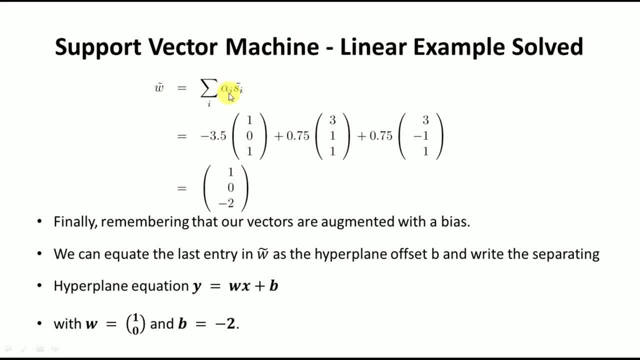 points. So how many nearest data points? we have in this case Three nearest data points. So this will become: i will be 3 alpha 1, s1 plus alpha 2 s2 plus alpha 3, s3.. So alpha 1 is. 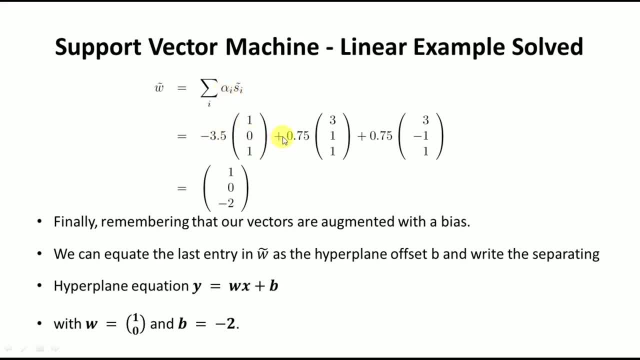 equivalent to minus 3.5,. s1 is 101 plus alpha 2 is equivalent to 0.75, alpha s2 is equivalent to 311 plus 0.75,, that is alpha 3.. s3 is equivalent to 3 minus 1, 1 here. So once you solve this particle equation, you will get: 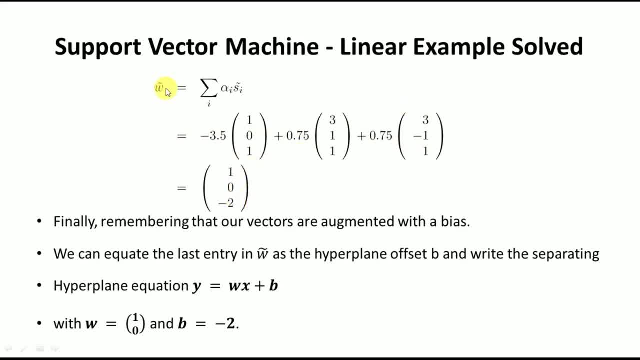 1, 0, minus 2 in this case. So w tidal, that is, w vector, is equivalent to 1, 0, minus 2.. So this one is after adding the bias. So now we need to differentiate bias and the actual. 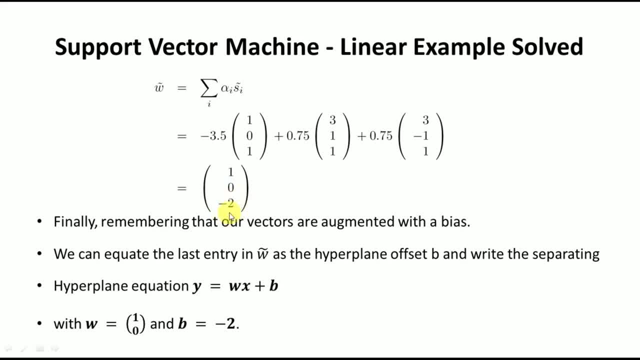 weight vector. So if you differentiate it, third one is always the bias here. So what we do here is the actual weight vector is 1, 0 and minus 2 is the bias in this case. So our line is: 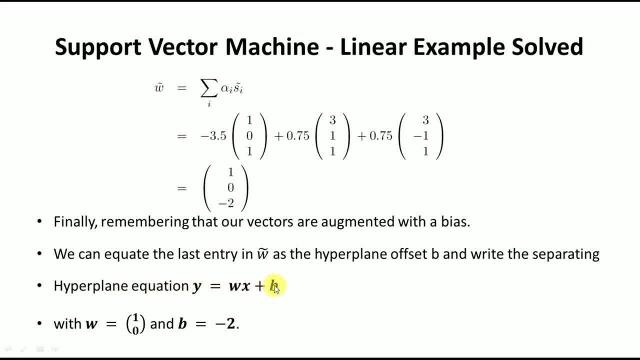 문 equation, or the hyper plane equation: y is equivalent to wx plus b, b is equal to minus 2 and w is equivalent to 1 and 0 here. So w is equivalent to 1, 0 and b is equivalent to minus 2.. So 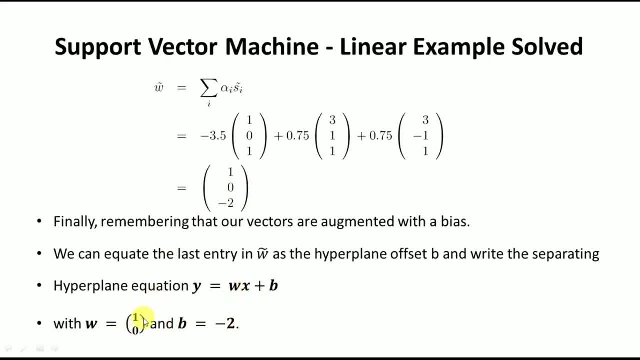 once you get this particular, the weight vector, we can decide what where the line should be drawn. because b is equivalent to minus 2, that is we need to consider. it should be either on the first quadrant, you can say: and w is equivalent to 1: 0. what is the meaning of 1, 0 is, x is 1, y is 0? it. 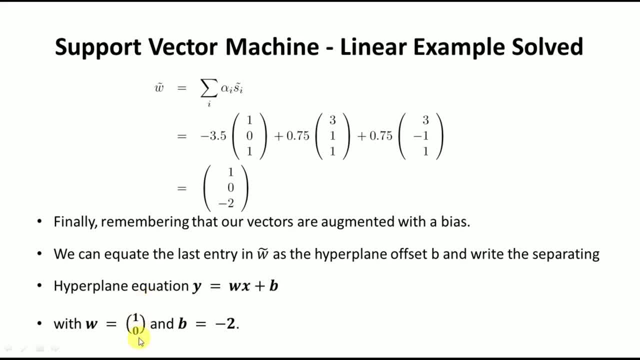 means that the line is parallel to y axis. if it is 0- 1, the line is parallel to x axis. if it is 1- 1, definitely the line will make 45 degree with respect to x and y axis. okay, so in this case, w is 1- 0, the line is parallel to y axis. so that is how actually we need to draw it. 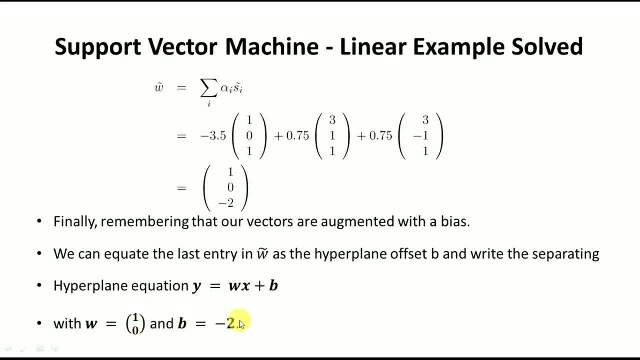 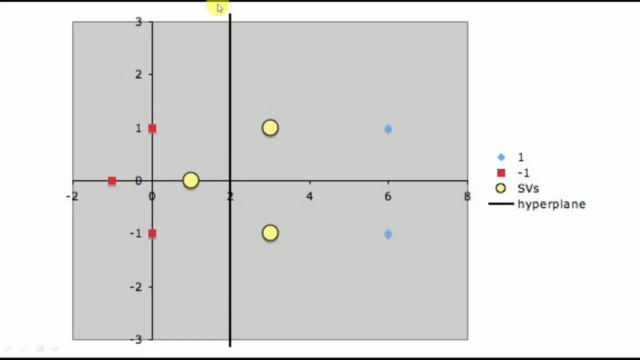 with a bias, or we can say that the offset is equivalent to minus 2. so if you look at this, one minus 2 means it should be in the first quadrant. either it will be over here or over here because the line is parallel to y axis. it will be considered here and then the line will.